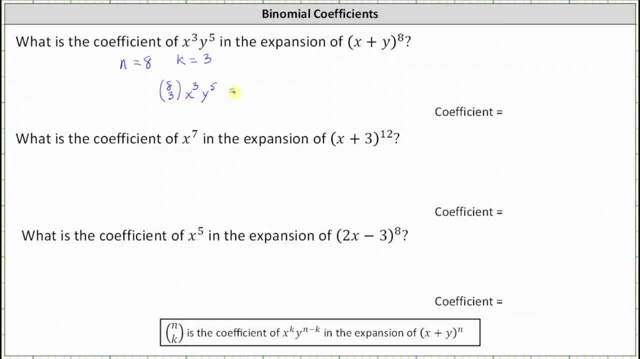 So this first example is very basic because it matches our notes perfectly, meaning the binomial is just x plus y. Eight choose three is equal to 56, and therefore the term is 56, x to the third, y to the fifth, and therefore the coefficient is 56.. 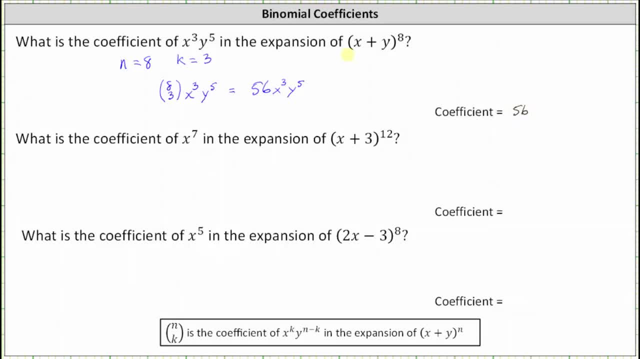 However, the coefficient is only 56 when we have a very basic binomial, like we have here, where the binomial is a sum of two variables and the coefficients are one. Many times this will not be the case, For example. the next question: 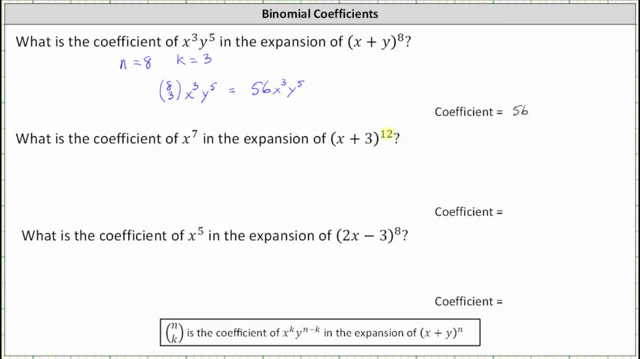 we're asked to find the coefficient of x to the seventh in the expansion of the 12th power of x plus three. Notice, in this case we don't just have x plus y, we have x plus three, which means for the note. 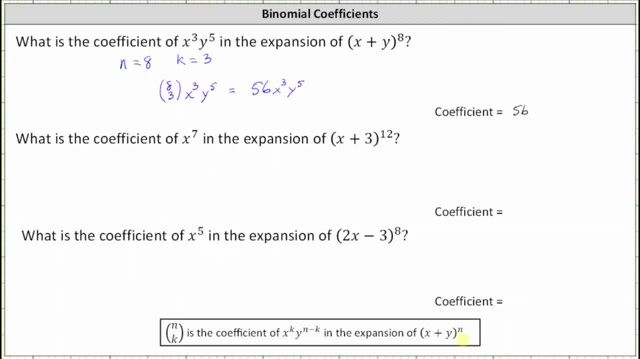 y is equal to three. But again, to begin notice, n is equal to 12.. And because we're looking for the x to the seventh term, we know k is equal to seven. So because the first term of the binomial is just x. 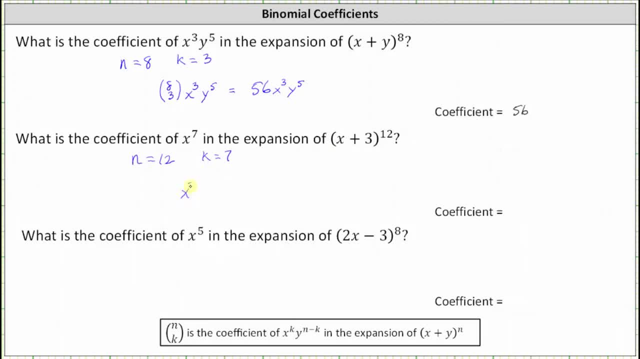 which matches our notes. the term is going to have x to the seventh in it, But then also notice, in our notes we have y to the power of n minus k. Our y value is positive three And therefore we have to multiply by three. 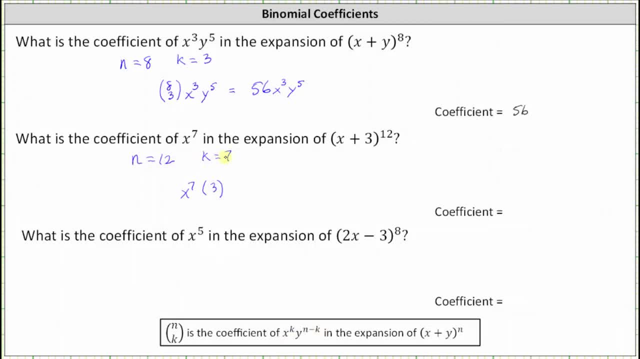 raised to the power of n minus k: 12.5.. 12 minus seven is five. The sum of these two exponents must always equal: n seven plus five is 12.. And then the combination is: n choose k, which is 12 choose seven. 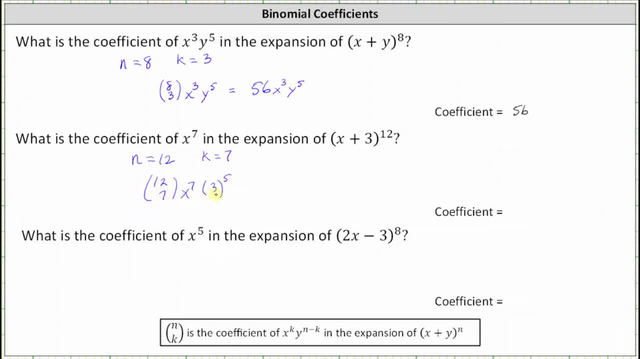 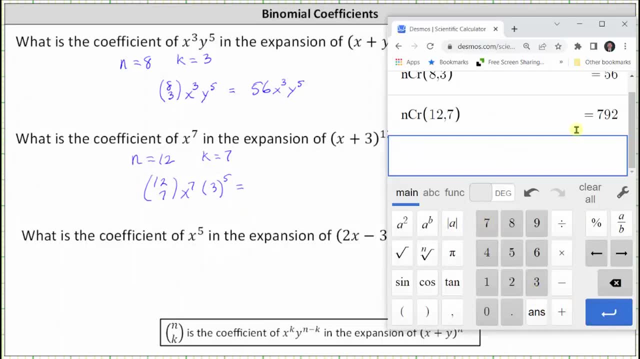 So notice, in this case, the coefficient is going to be 12, choose seven, times three to the fifth. So let's go ahead and work this out. Let's determine 12 choose seven, which is 792.. And three to the fifth is equal to 243.. 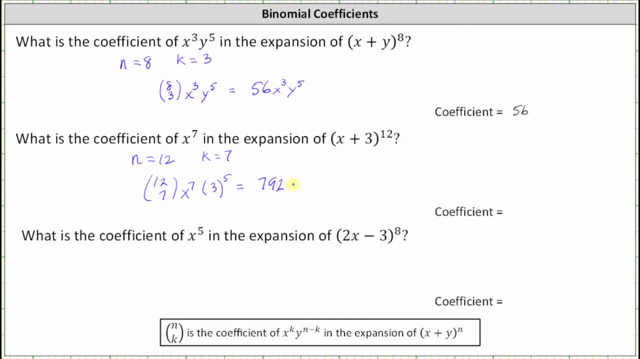 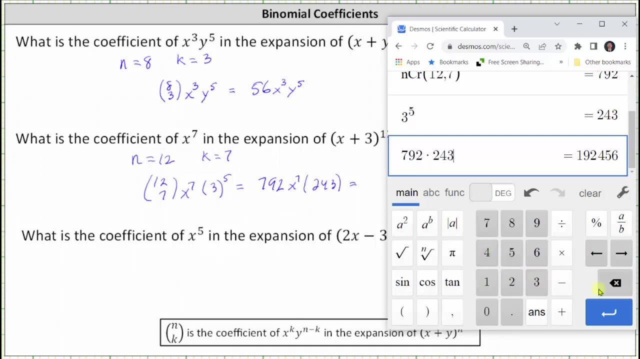 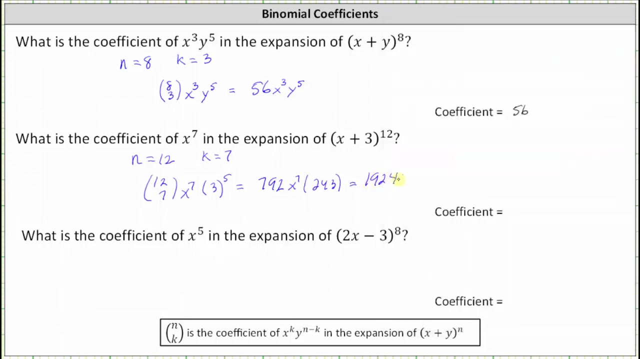 So here we have 792 times x to the seventh times 243.. So the term is 792 x to the seventh times 243, which is 192,456 x to the seventh, And therefore the coefficient is 192,456.. So notice here. 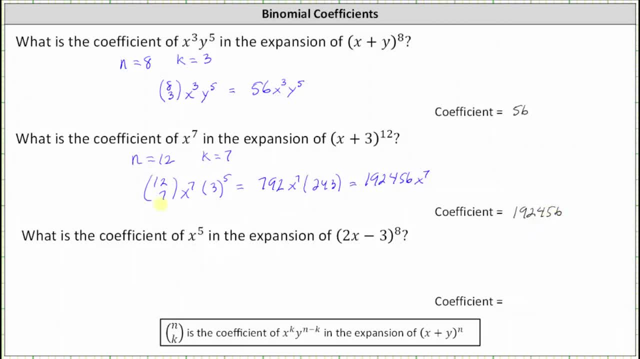 this is more common, where the combination is not the ending coefficient, but we do need it to determine the coefficient. And then, for the third example, we're asked: what is the coefficient of x to the fifth and the expansion of the eighth power of two x minus three?